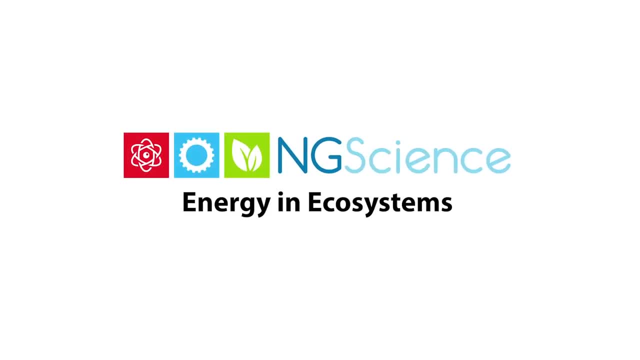 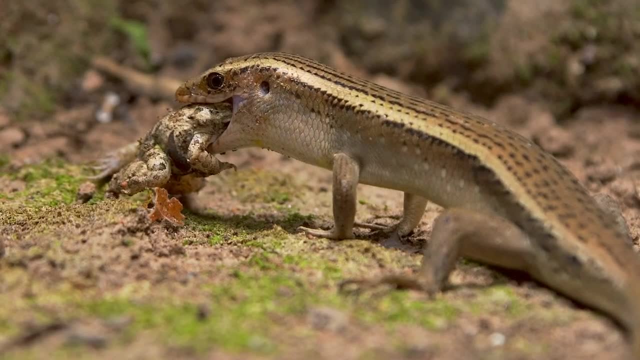 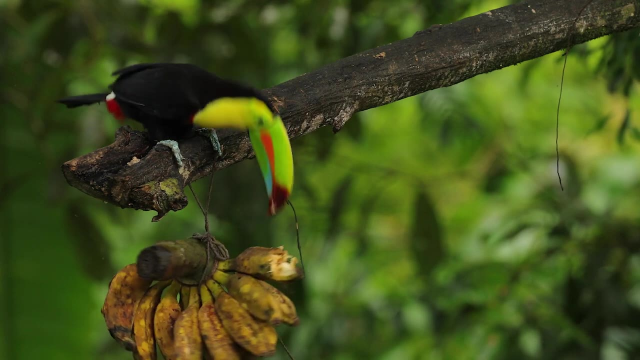 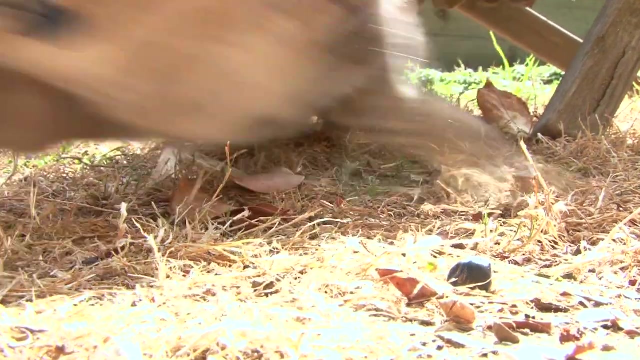 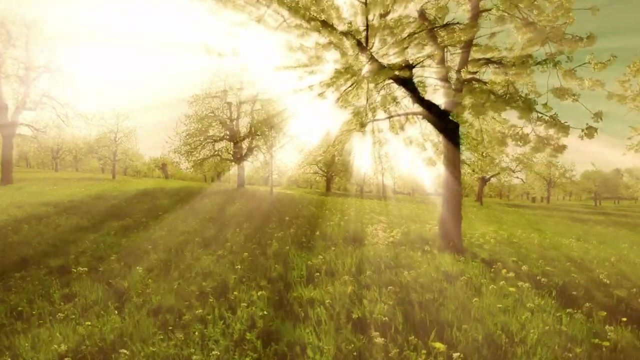 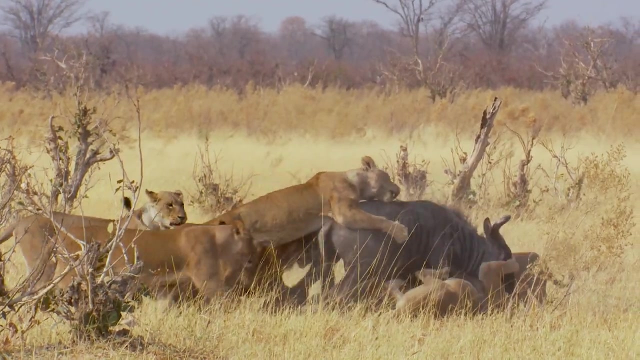 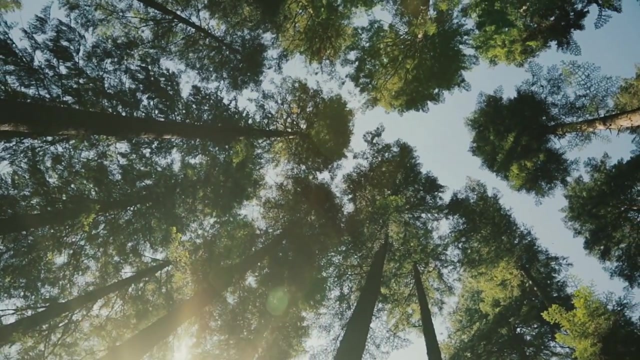 All of the organisms in an ecosystem need energy, And different organisms get the energy they need in different ways. Some make food through photosynthesis, Some eat other organisms, Others break down the remains of dead plants and animals. How an organism gets its energy determines the role it plays in an ecosystem. 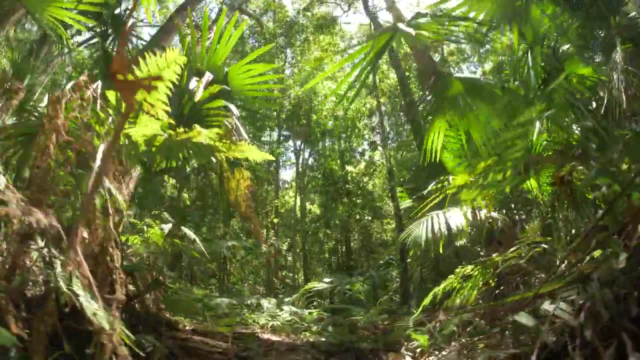 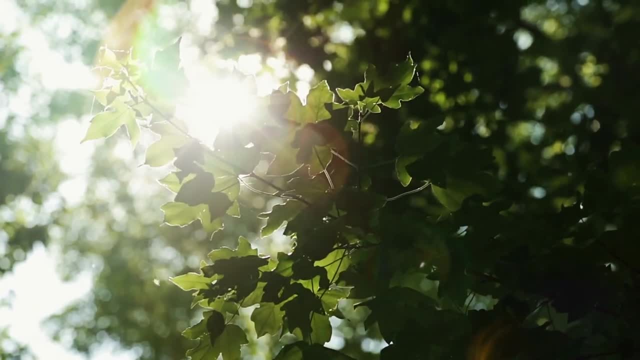 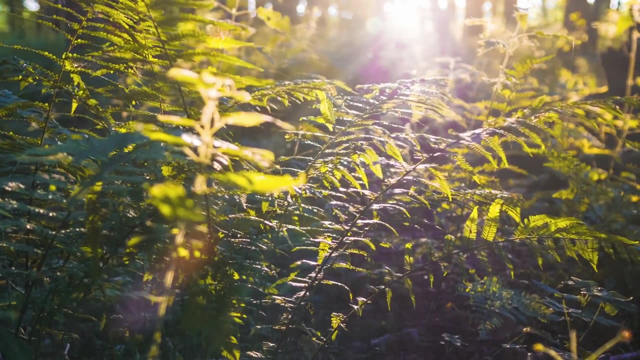 An organism that makes food through photosynthesis is called a producer. In most ecosystems, plants are the main producers. They use light energy from the sun, carbon dioxide from the air and water in the soil to produce food in the form of sugar. 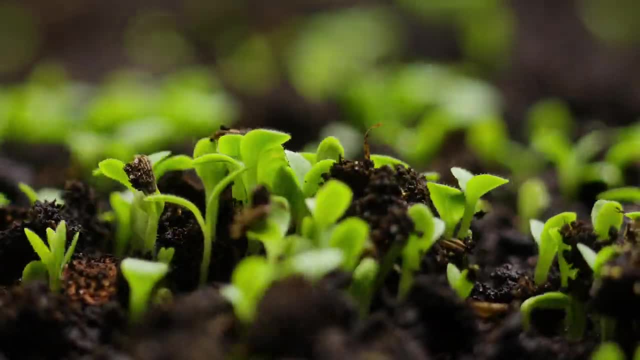 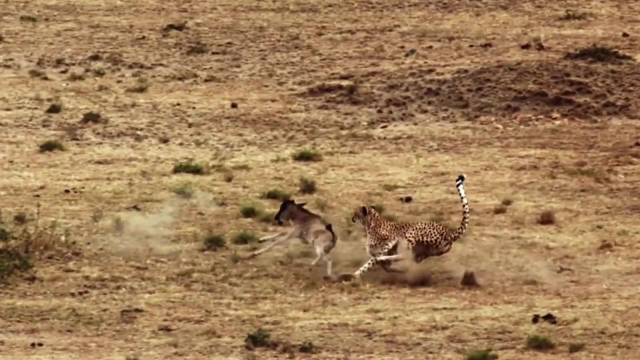 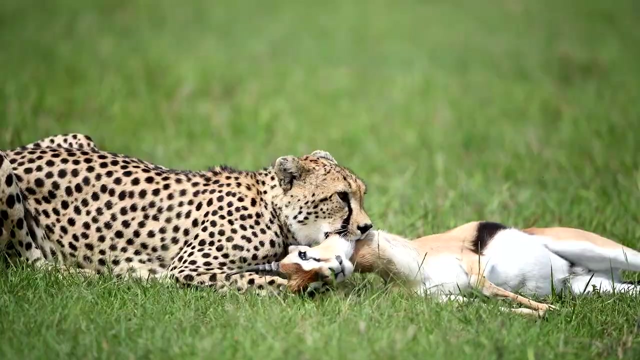 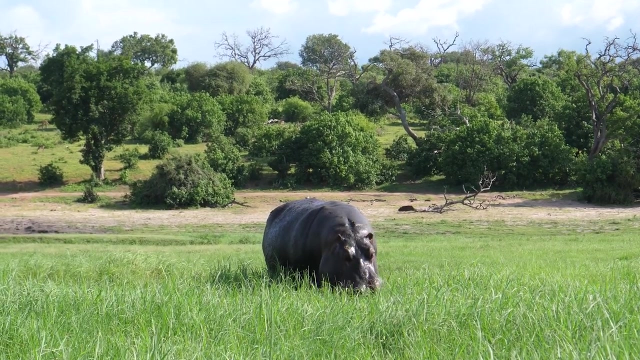 During this process, they also give out oxygen. An organism that gets energy by eating other organisms is called a consumer. All animals are consumers. They get the energy they need by feeding other organisms in the ecosystem. Animals that eat only plants or plant parts are called herbivores. 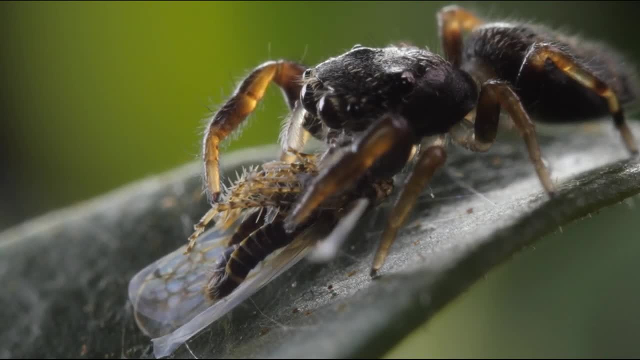 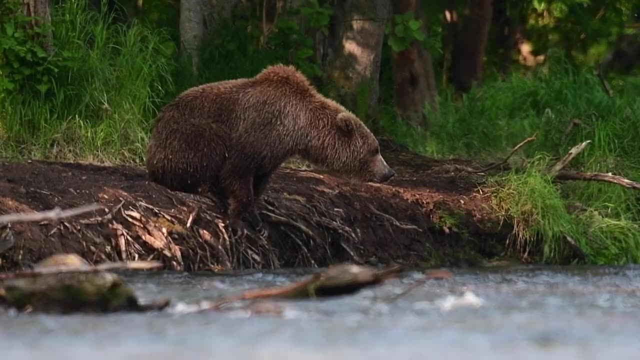 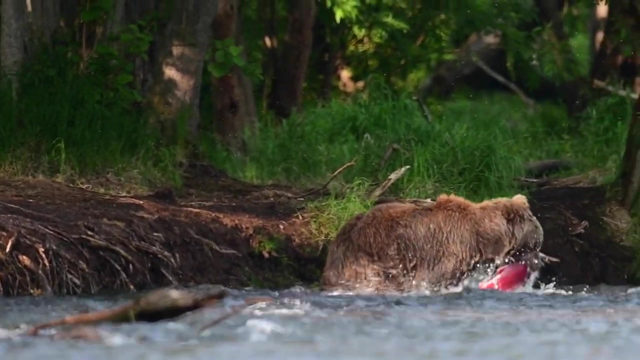 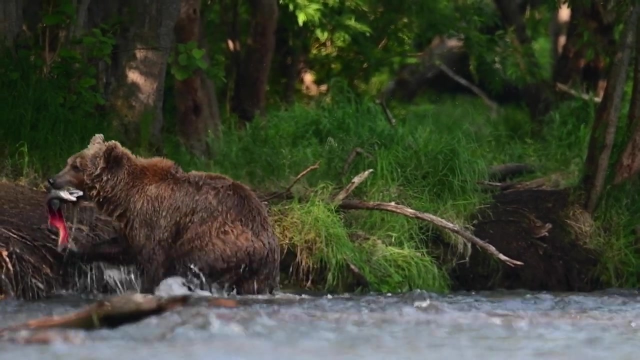 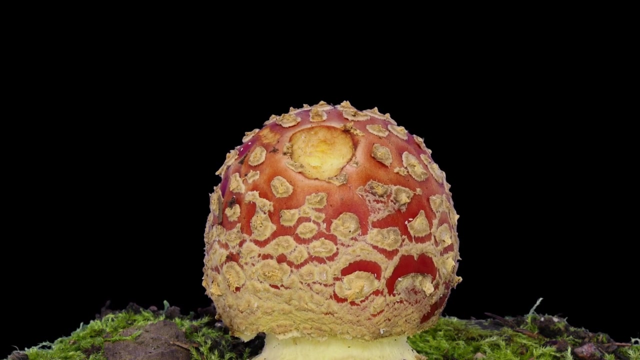 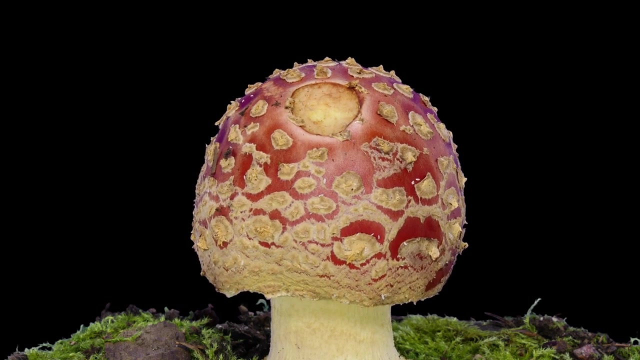 Those that eat only other animals are carnivores, And those that eat both plants and animals are called omnivores. I guess that makes me an omnivore. Some organisms meet their energy requirements by breaking down or decomposing the remains of dead plants and animals by feeding on the broken down material. 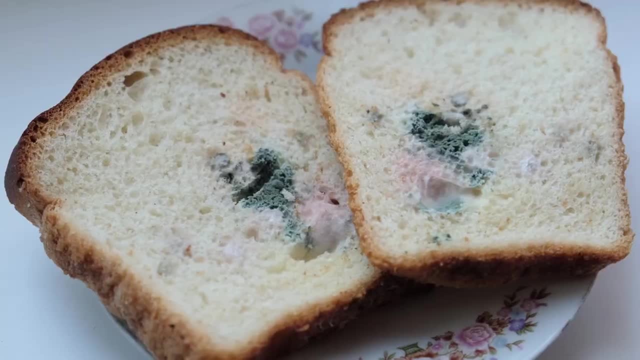 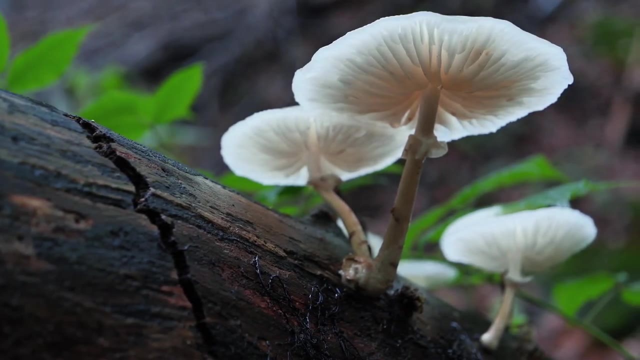 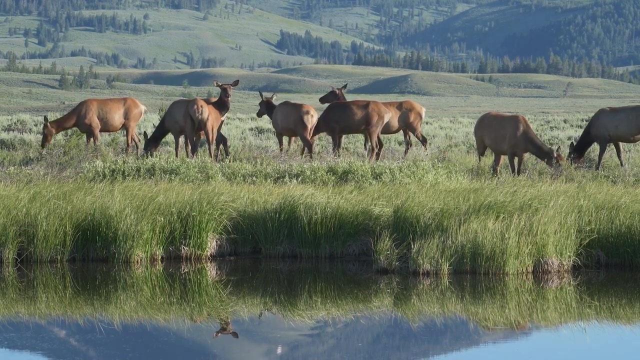 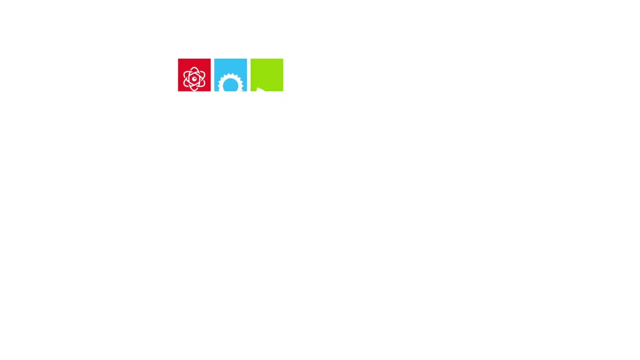 These organisms are called decomposers. Bacteria and fungi are decomposers. Decomposing releases nutrients back into the ecosystem. Wander around an ecosystem in your area. See what producers, consumers and decomposers you can spot. See ya. 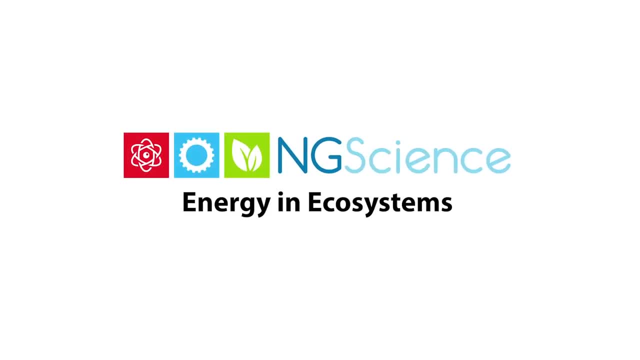 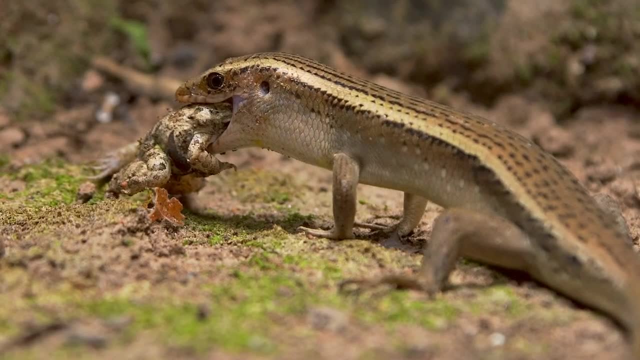 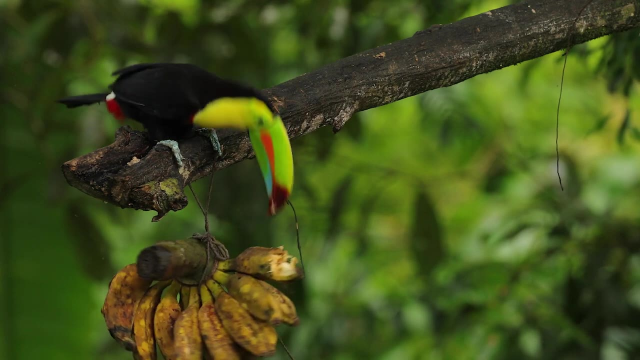 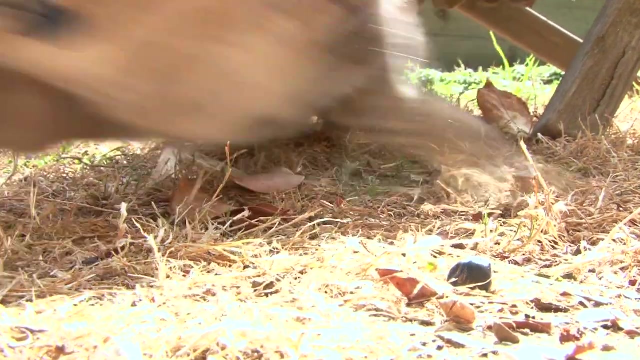 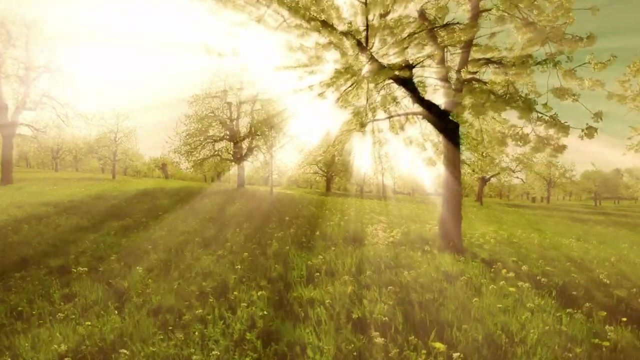 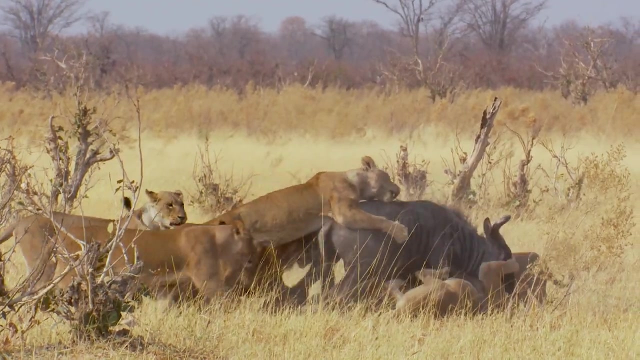 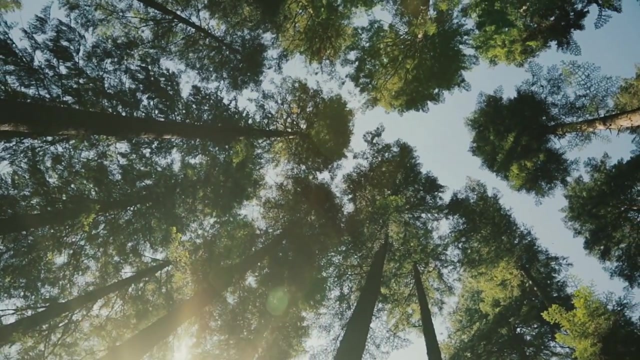 All of the organisms in an ecosystem need energy, And different organisms get the energy they need in different ways. Some make food through photosynthesis, Some eat other organisms, Others break down the remains of dead plants and animals. How an organism gets its energy determines the role it plays in an ecosystem. 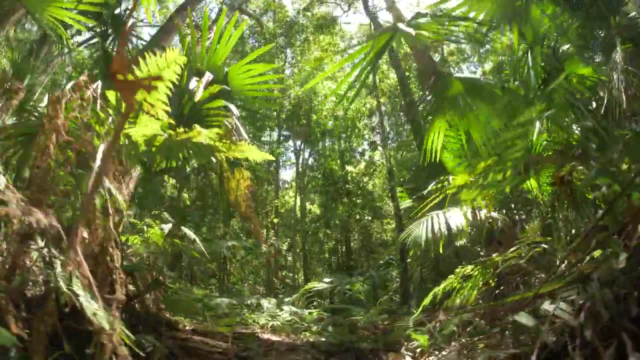 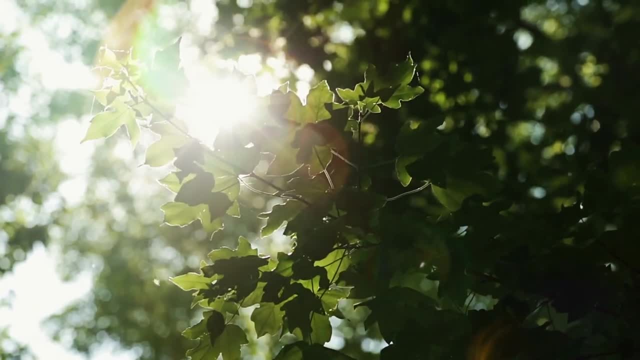 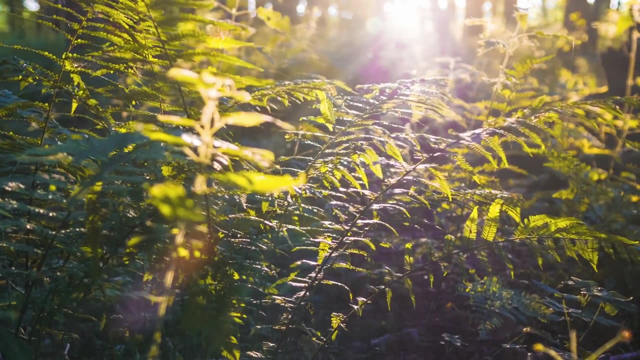 An organism that makes food through photosynthesis is called a producer. In most ecosystems, plants are the main producers. They use light energy from the sun, carbon dioxide from the air and water in the soil to produce food in the form of sugar. 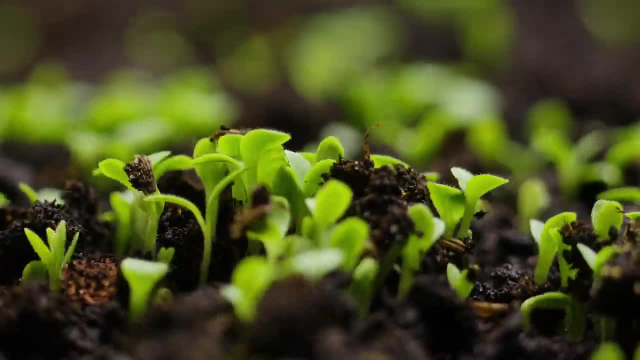 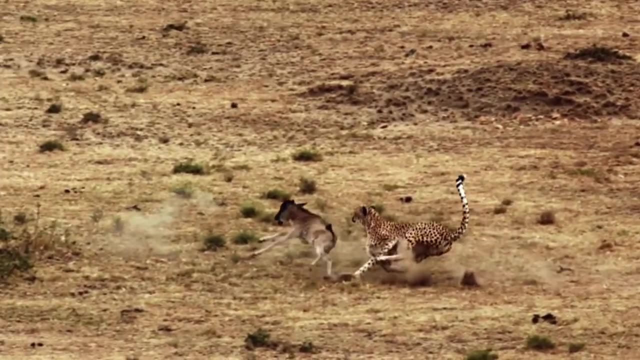 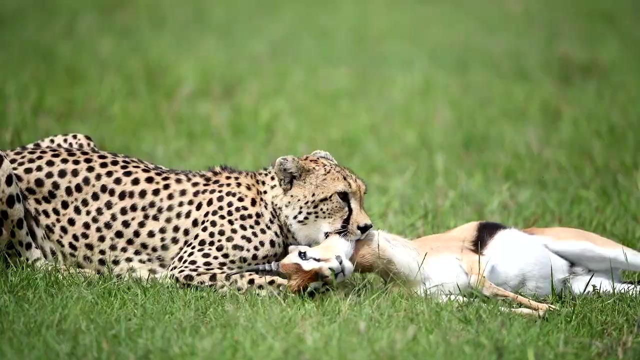 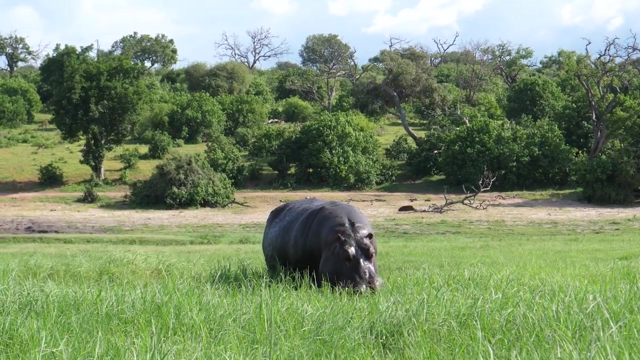 During this process, they also give out oxygen. An organism that gets energy by eating other organisms is called a consumer. All animals are consumers. They get the energy they need by feeding other organisms in the ecosystem. Animals that eat only plants or plant parts are called herbivores. 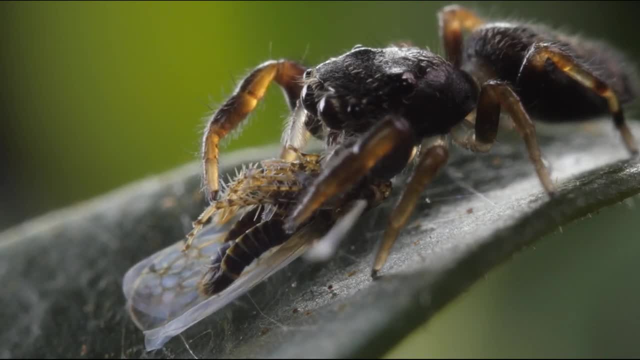 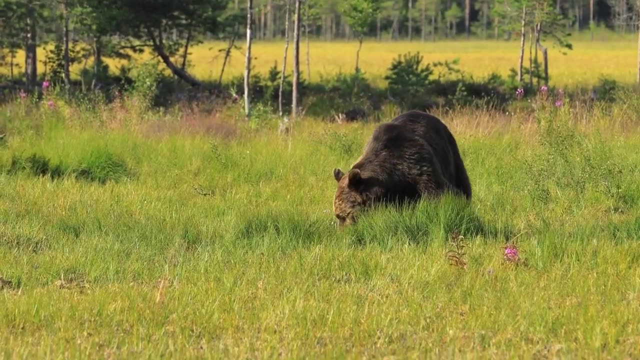 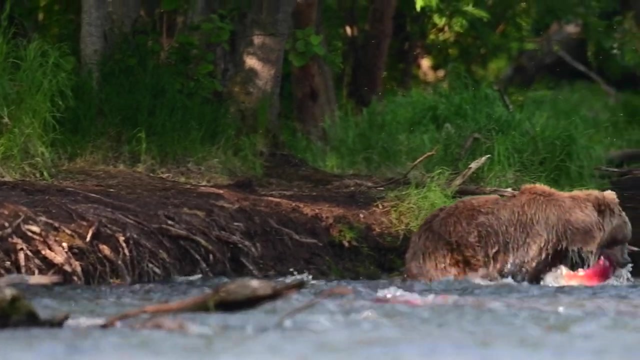 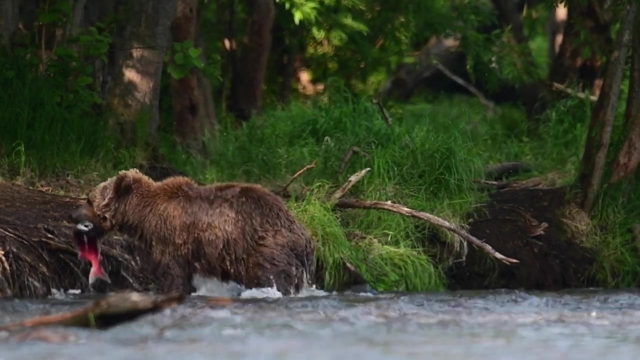 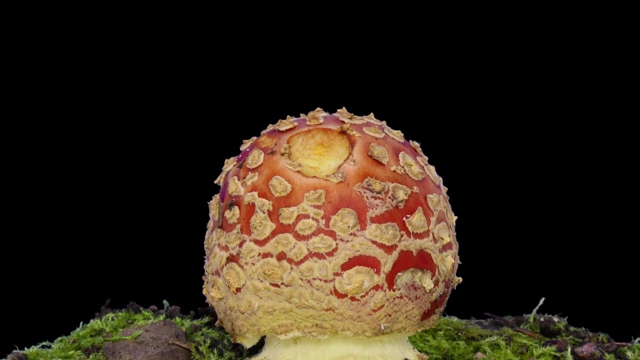 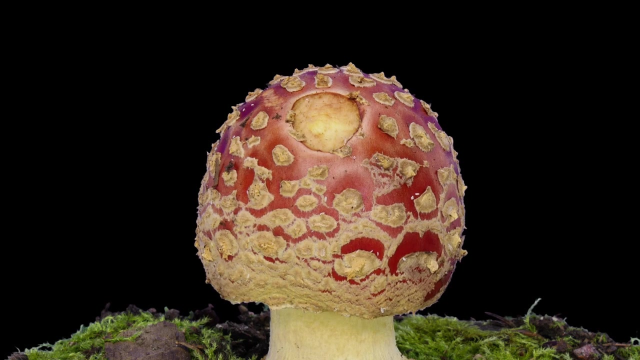 Those that eat only other animals are carnivores, And those that eat both plants and animals are called omnivores. I guess that makes me an omnivore. Some organisms meet their energy requirements by breaking down or decomposing the remains of dead plants and animals by feeding on the broken down material. 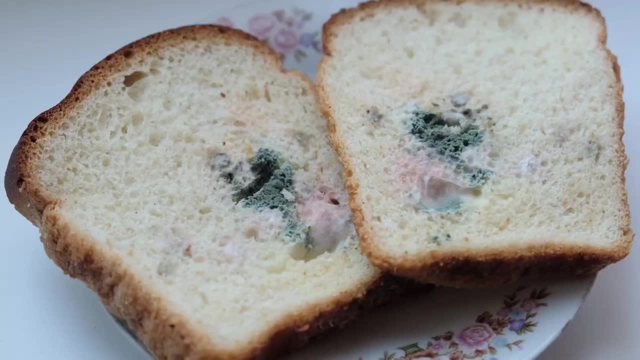 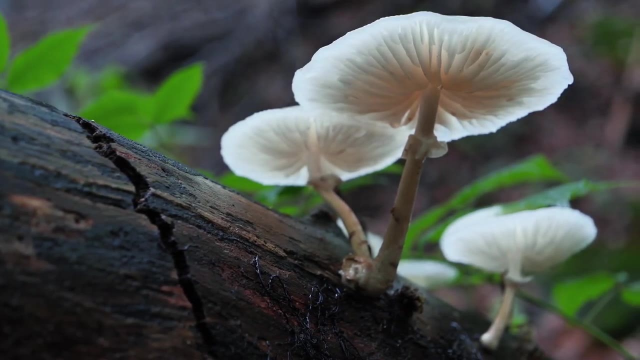 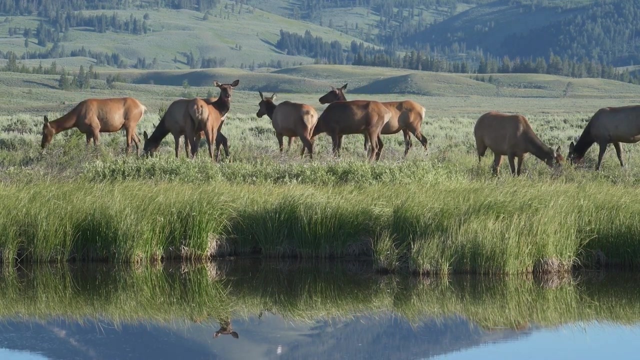 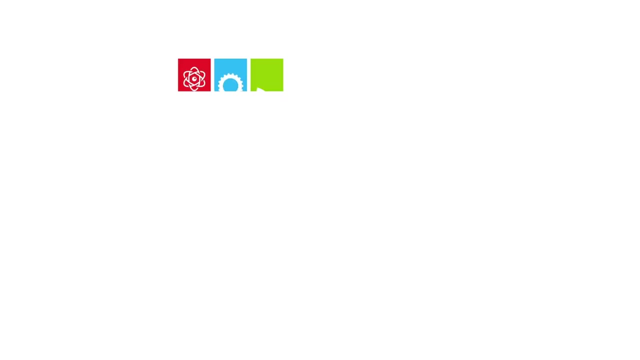 These organisms are called decomposers. Bacteria and fungi are decomposers. Decomposing releases nutrients back into the ecosystem. Wander around an ecosystem in your area. See what producers, consumers and decomposers you can spot. See ya.